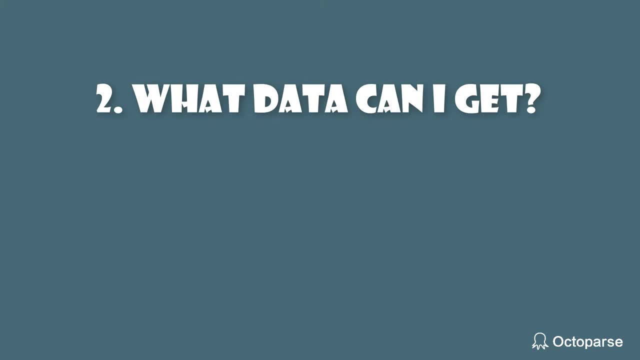 Well, you may want to know what data can I get? with web scraping, You can get price data of a set of products from an array of target websites. With the data at hand, you can easily spot the lowest-priced product, the highest-priced product. 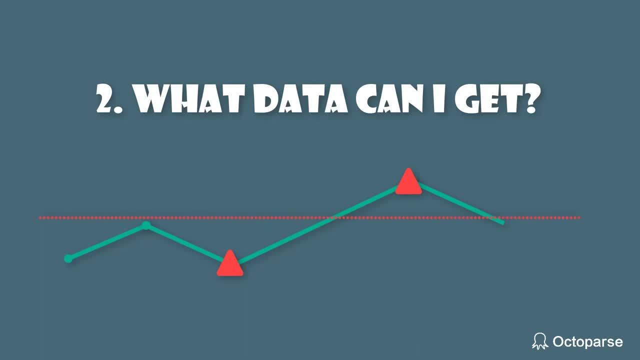 the lowest-priced of a product, the average pricing of them, or the average price of one of them over a span of time. Put it simply, you just get all price data of all products you are interested in. So how can this data help generate high profits? 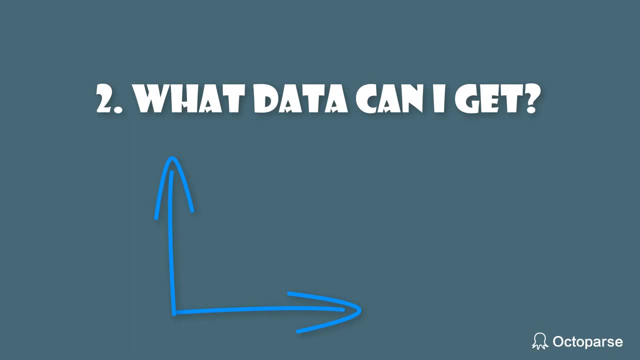 Our users just build a model from the data. Say X represents the price and Y the sales. They get an algorithm out of it and choose the best mix as their pricing strategy With which they would get the maximum profits. If you know nothing about this sort of price comparison model, search on YouTube. you can get a lot of tutorials. 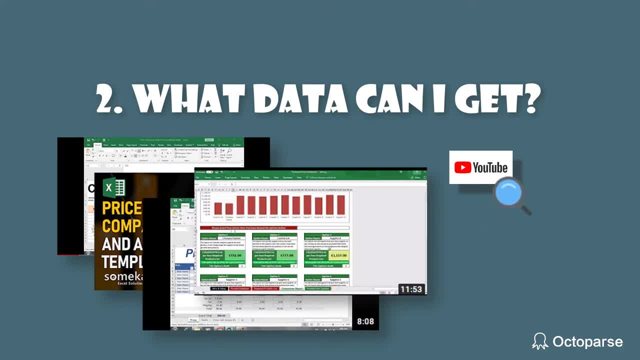 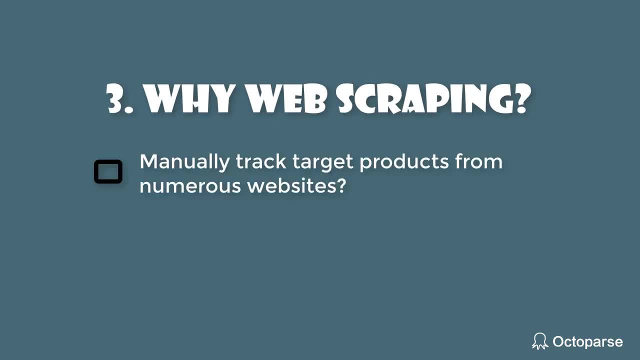 like price comparison model in Excel and pick it up quickly. So why web scraping? First, it is self-evident that tracking the prices of products on numerous websites manually is just not applicable. You need a tool. Second, with raw data that is accurate, you can make anything out of it. 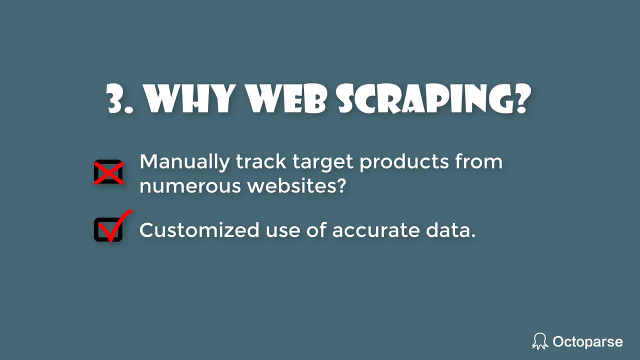 There is no constraint in use and no sacrifice in the data quality. Last, just keep up with your peers. They are acting upon your strategies. You should mind their tricks too. Let's come to the last part: how to use Octopus to get data for price comparison. 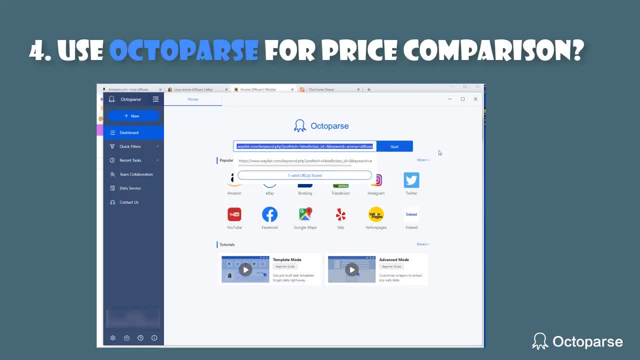 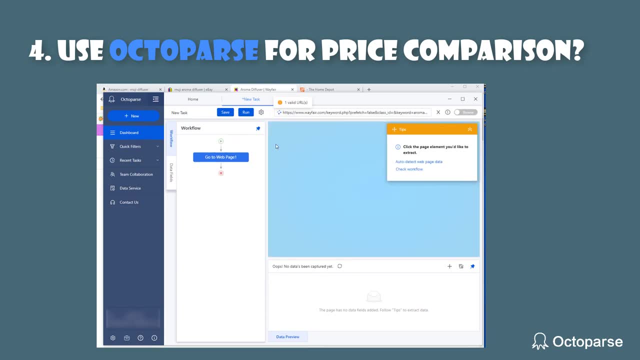 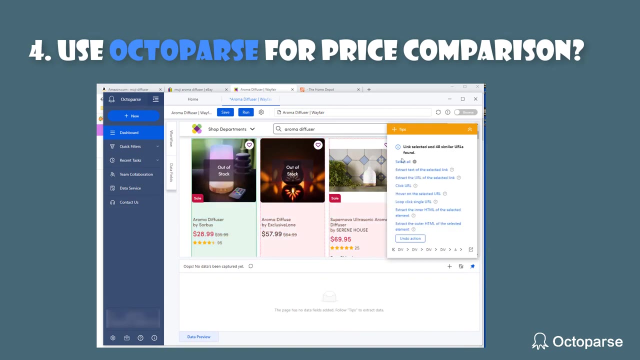 This is a small demo of how I use Octopus to scrape from Wayfair. Enter the URL you want to scrape from. Wait for it to load a bit. Click the product cards. Click one of them And select all. In this way, all products are selected.